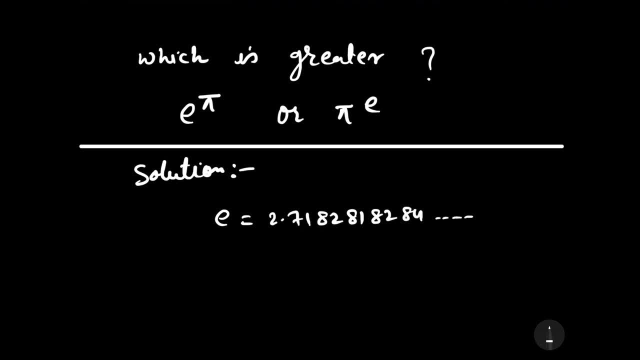 till infinity, since it is a irrational number and pi is also an irrational number, you all know that, and its value is 1415926 and some more digit. if you want to take that, Both are the irrational number. if you want to calculate it manually, then you will not. 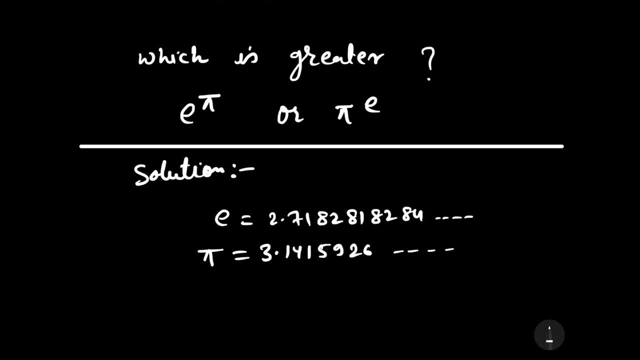 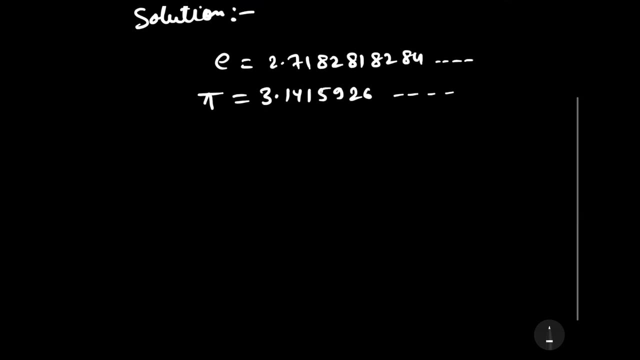 be able to solve it manually. but obviously you can calculate it by calculator. but point is that we are not interested to calculate it by calculator, we want to solve it by some other means. I will try to solve it by the two different method, which will be very easy. 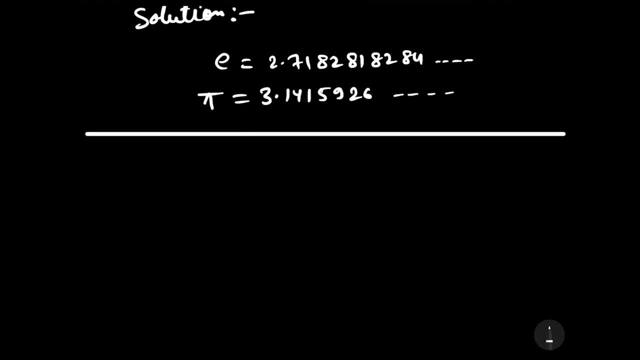 one. let me solve it by the method. one Method first, let us draw the graph of function y is equal to 1 by x. the graph of function y is equal to 1 by x is look something like this for positive quadrant of x and clearly. 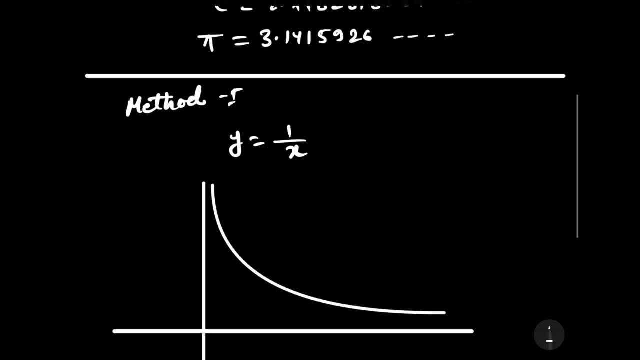 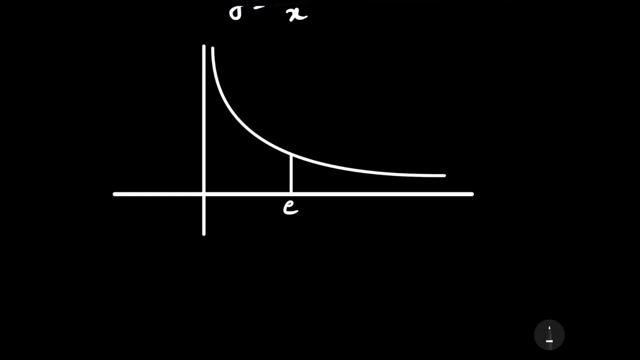 you have seen that the value of pi is greater than the value of e, then the value of. if you will put e, then this will be here and the value of pi will be here. if you want to calculate the area of this region, then we can calculate it by the method of integration. so let us. 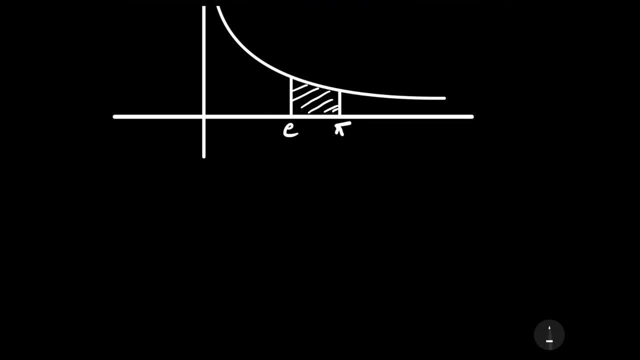 calculate the area of this shaded region, then this can be calculated by integration 1 by x into dx, from e to pi 's, by integrating it, the integration of 1 by x into d x is log base, e log base, e x from. 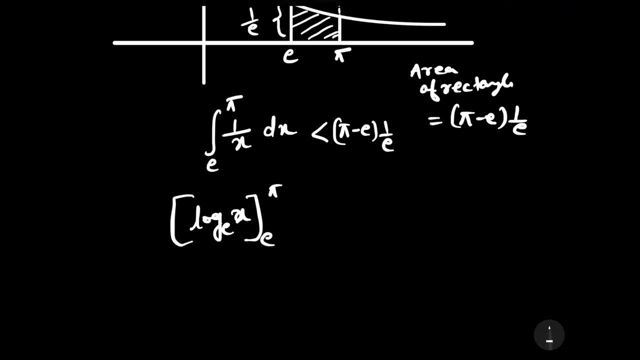 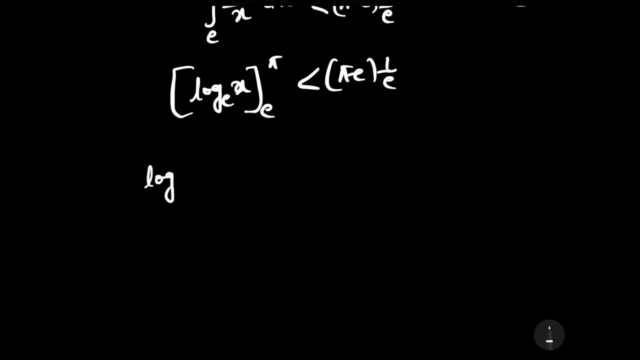 e to pi, which will be less than pi minus e times. well, pi minus e times of 1 by e. further we can hold, further we can solve it by putting the limit log e base, pi minus log e, bar minus log e base e, which will be smaller than pi minus e times of 1 by a. But we know that. 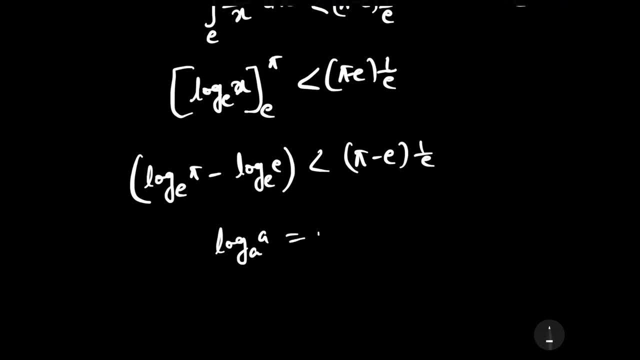 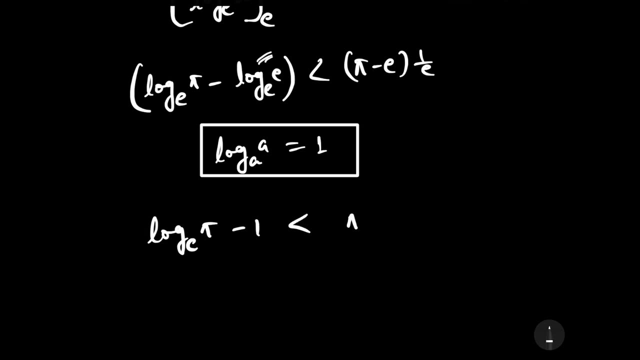 log a base a is equal to 1. with help of this formula, we can put the value of log e base e is equal to 1.. Therefore, we can write log e base pi minus 1 will be smaller than pi minus e into 1 by e. Further, we can write it as log e base pi minus 1 will be less than. 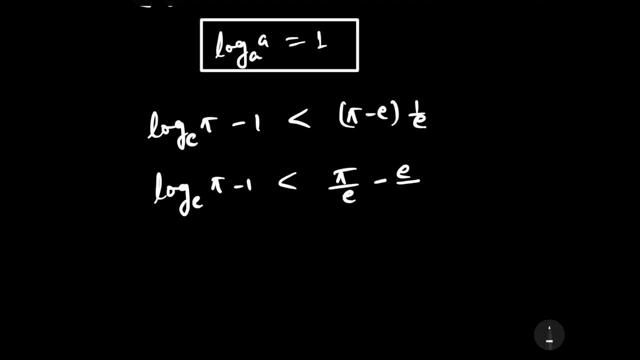 pi by e minus e into e by e And further it can be written as log e base pi minus 1, which will be less than pi by e minus 1.. Minus 1 will be cancel out with minus 1 of RHS side by adding plus 1 and plus 1.. Therefore we can write it as log e base pi. 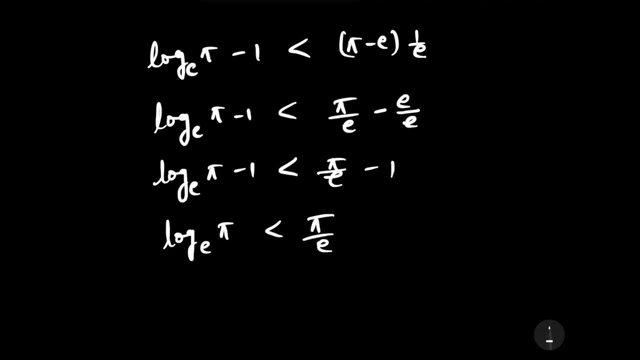 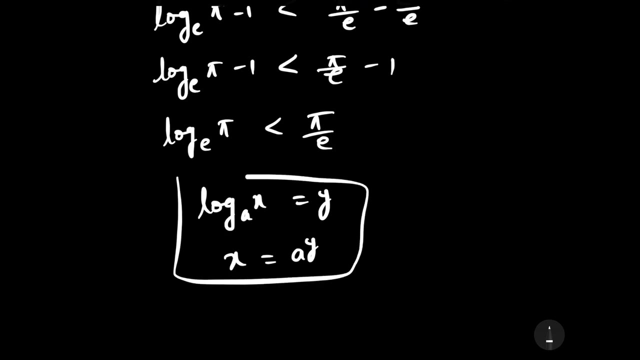 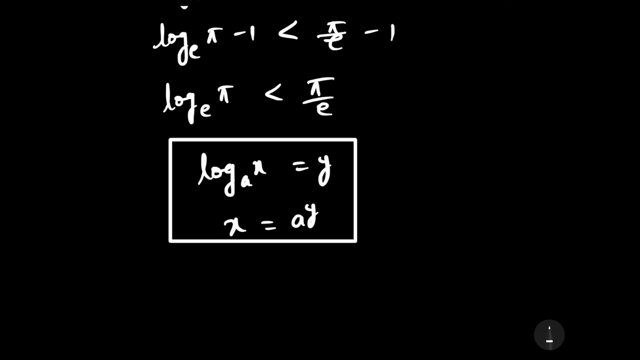 will be less than pi by e. Further, we can say that log a base x is equal to y. then this can be written as: So x is equal to a to the power y. this is the formula. with help of this formula we can write no. first of all, let us multiply it by e on both side. 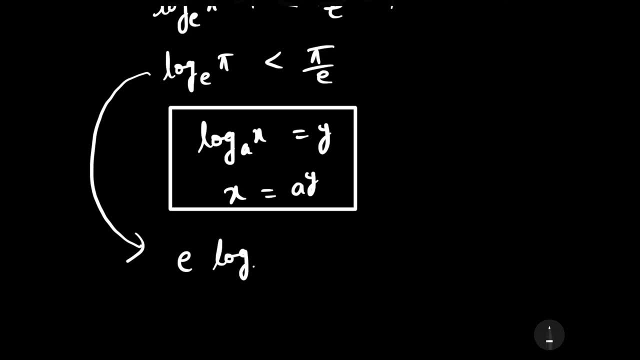 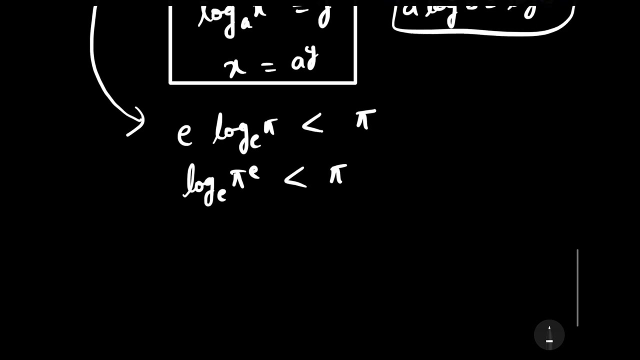 Then this will be equal to e. log e base pi will be less than pi. and we know another formula of log, that is a log b can be written as log b to the power a. With the help of this formula we can write log e base pi to the power e will be less than pi and further we: 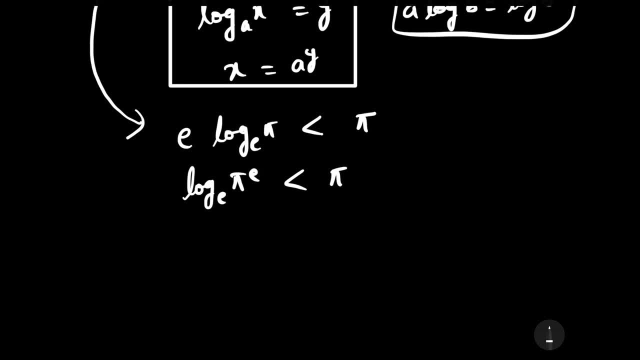 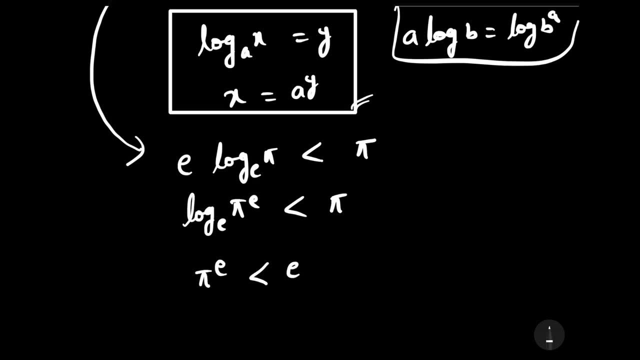 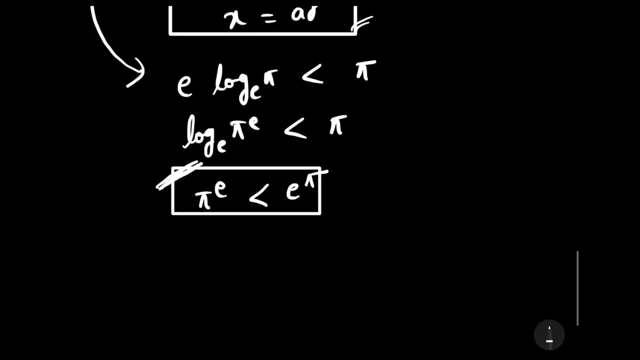 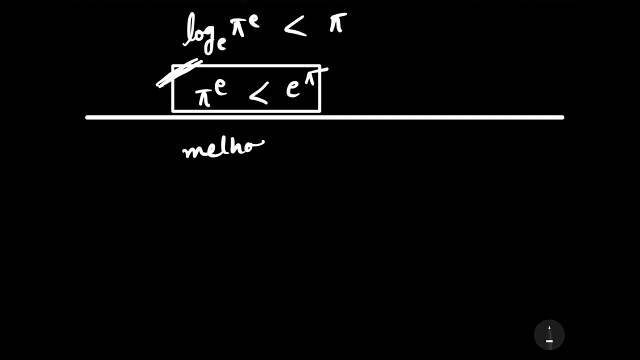 can write it as: with the help of this formula, we can write it as: So: log e base pi to the power e will be less than e to the power pi, and this is our required answer. Now let us solve it by another method, that is, the method number method second to: 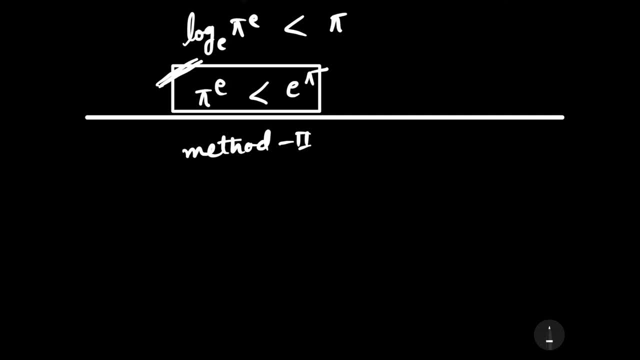 solve it by method. second, we should know the Taylor series expression of e to the power x by Taylor series can be expanded to: we can write it as: 1 plus x plus x square by 2 factorial plus x cube by 3 factorial till infinity. From this expansion we can clearly say that 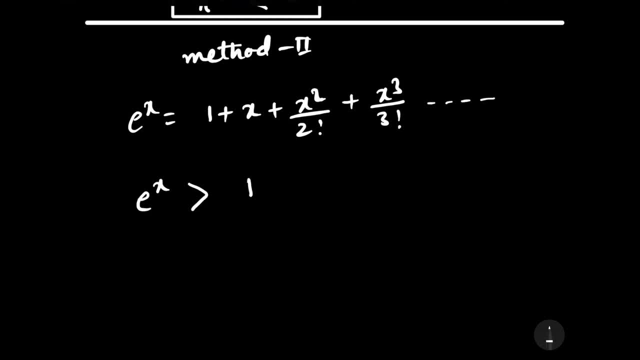 e to the power x will be greater than the partial sum of 1 plus x, since this is equal to this large number of summation, but e to the power x will be greater than this partial summation, since we are taking only 2 term. Therefore, e to the power x will be greater. 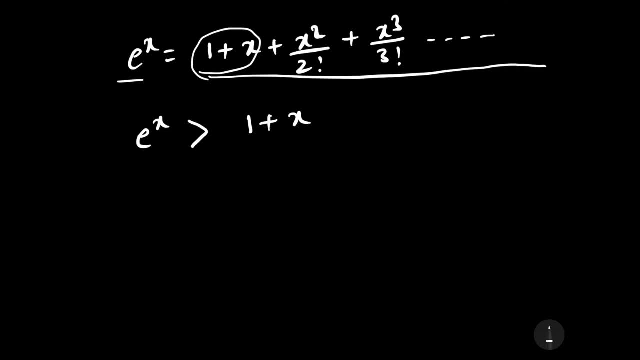 than 1 plus x. Now let us take a intelligent choice. that is, value of x is equal to pi by e minus 1. to prove our questions, yet to solve our questions solution: Now let us put the value of x, e to the power. pi by e minus 1 will be greater than 1 plus. 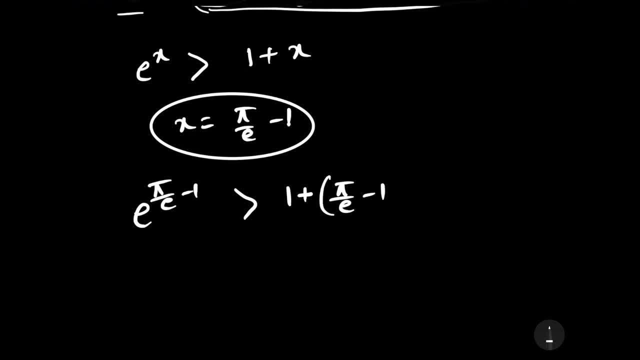 pi by e minus 1.. This is the value of x. further we can write e to the power. pi by e into e to the power minus 1 will be greater than pi by e, and further it can be written as e to the power pi. 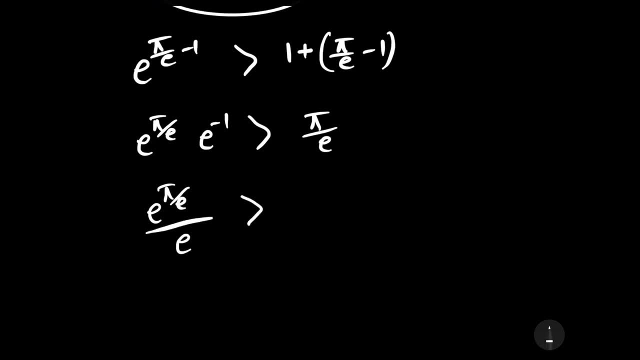 So if c is e to the power pi by e divided by e greater than pi by e, multiplying both side by e, we will have e to the power pi by e will be greater than pi. now raise both side a power e, then we will have e to the power pi by e to the power e will be greater. 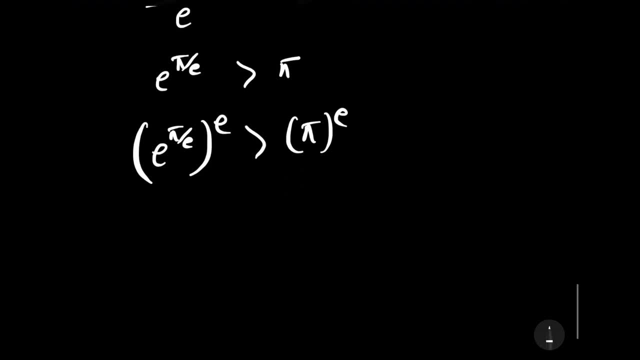 than pi to the power e, and we know that if there is a e to the power m multiplied by n, then it can be written as a to the power m into n. with help of this formula we can write it as pi by e into e will be greater than pi to the power e and this is equal to e to the power pi. 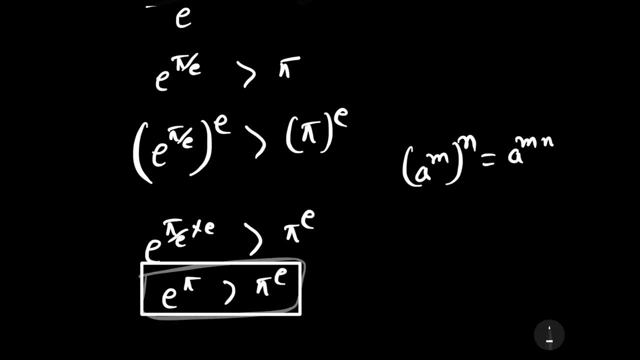 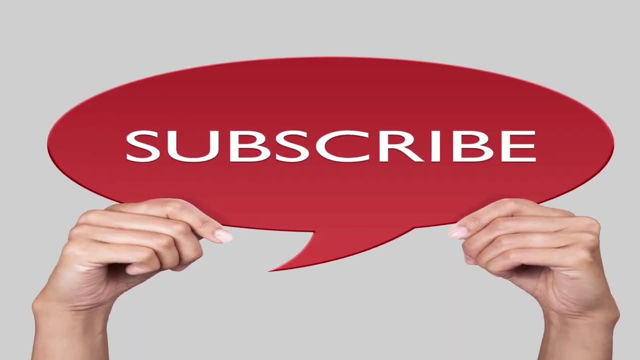 greater than pi to the power e, and this is our required solution. Thanks for watching this video. don't forget to like, comment and share. please subscribe our channel to support us and thanks once again. Subtitles by the Amaraorg community.